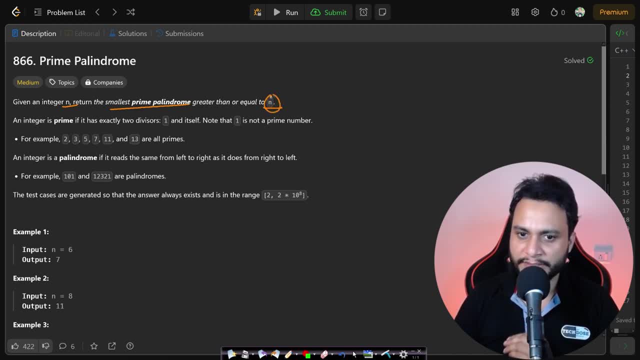 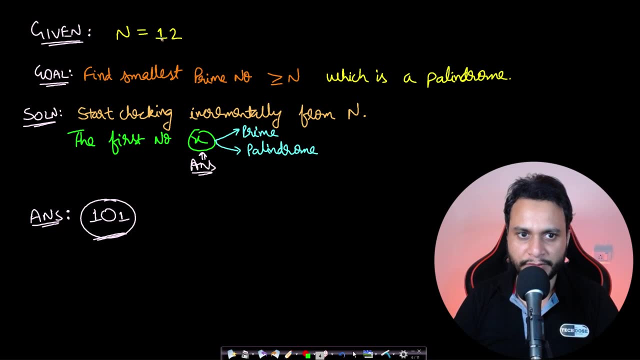 n. So the number should be a prime number, It should be greater than equals to n and it has to be a palindrome. Let's look at an example for better understanding. Let's say that our given n value is 12.. Okay, now we need to find the smallest prime number, which? 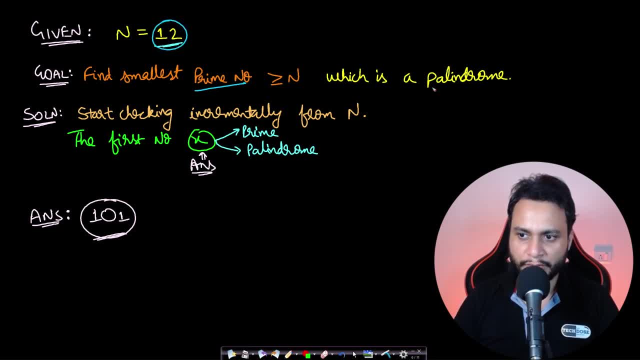 is greater than equals to 12 in this case, and it should also be a palindrome. So the solution is to start checking incrementally in steps of size one from n, that is, we will first check for 12 if this is a prime number or not a prime number, If it happens to be. 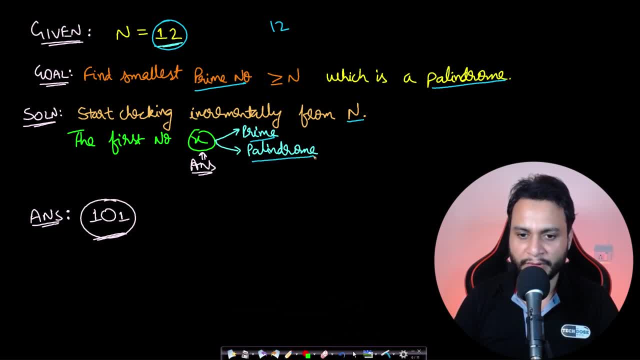 a prime number, then we have to check if it is a palindrome number or a non palindromic number, right? So the first thing is the number should be a prime number and then it has to be a palindrome as well. So in this case, if we start checking from 1213, 13 is a prime, but it is not a palindrome. again 14 and so on. If you keep on going, then we will find that 101 is the first number we encounter, which I mean when we started checking from 12.. This is the first number, which was prime as well as a palindrome. Okay, so the answer in this case is 101.. Now in. 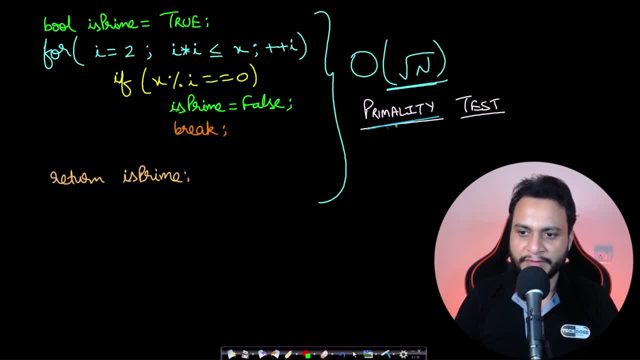 order to solve this problem, the first thing we should know is how to check if a given number is a prime number. So if you want to check primality for a number x, then we have to just run from two to square root of x. 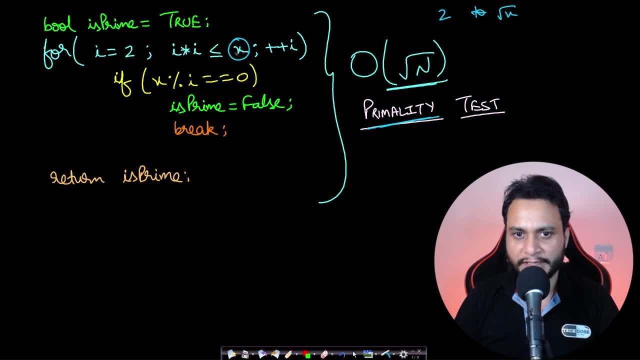 right And you can write it as i equals two to i into i less than equals to x, which is basically going to square root of x in steps of size one, And if any number can divide the given number x, then it is a non prime number. otherwise it will be a prime number. 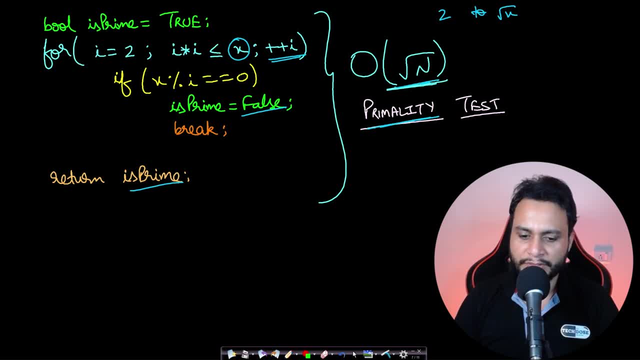 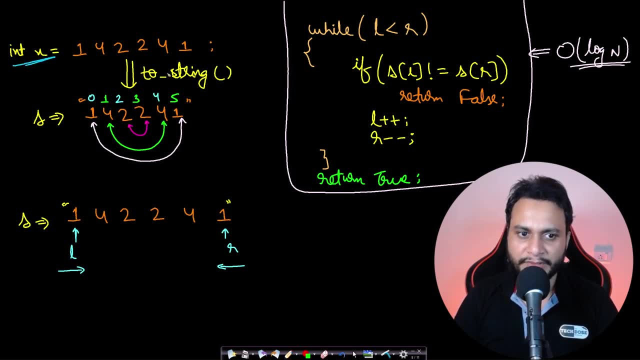 Fine, So this can be done in order of root n time. So once you are done with the primality test, the next thing to know is how to check for a palindrome, And this is also very easy. Given an integer number, we can simply convert it to a string, And once we know the string, 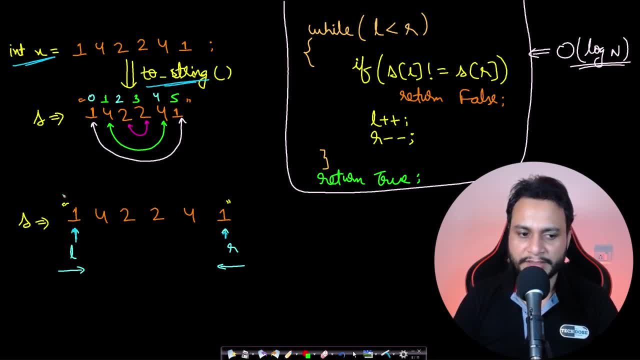 then we can use the two pointers, left and right, And we can start checking from both the ends. So your left should be equals to right. if it is equal, then move your left to the right and move your right to the left and again, keep on checking, Keep on checking. 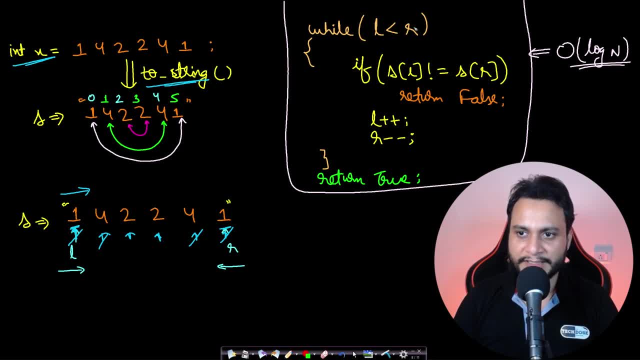 unless this L becomes equal to 0.. comes equals to r or l exceeds r. okay, and this is a simple code to check if a given string is a palindrome or a non-palindrome, using two pointers, and here is a diagram for the given example, like: 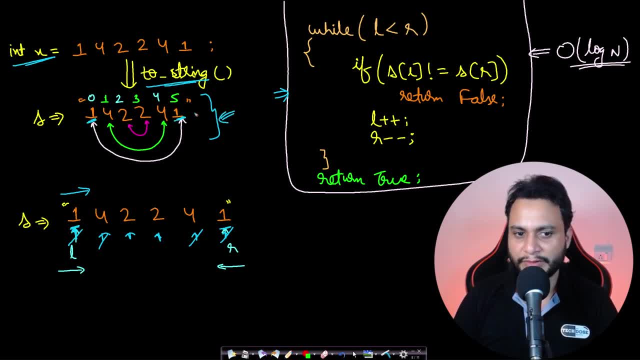 this last character on the left side should be matched with the last character on the right side. second last on the left side should be matched with second last on the right side. fine, so this can be done in order of log n. why log n? because n was actually the integer. okay, so here this is an. 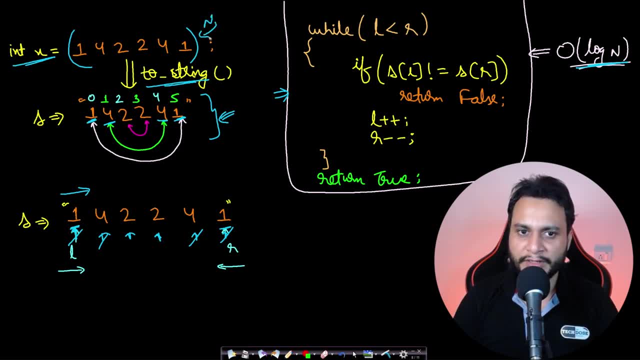 integer number 14, 22, 41, so this is equals to n. but when you convert to the string, the length of the string is equals to the number of digits in this integer right. so the number of digits will be log n base 10, because this is a base 10 number system and therefore the length of the string is 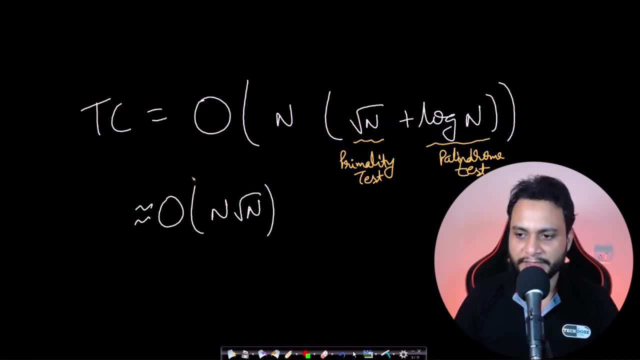 log n. now, once we know about the primality test and how to find a palindrome, you know that we have to repeat it for a lot of numbers. so i'm just taking an n factor here. obviously it can be less or greater than n, but let's take it n. that is the number of times we will be running. 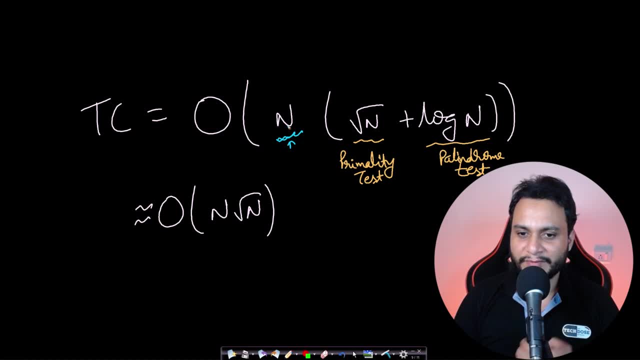 the checks. so there is no bound to it because we are checking from n and going beyond that point. but it will not be a very large gap. so the primality test takes root n time and the palindrome test will actually take log of n time. therefore we can come to a conclusion of n root n. 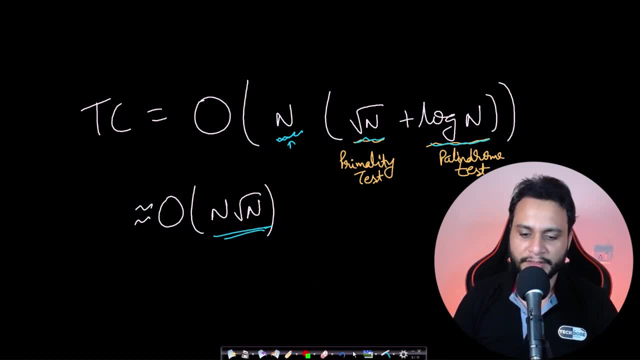 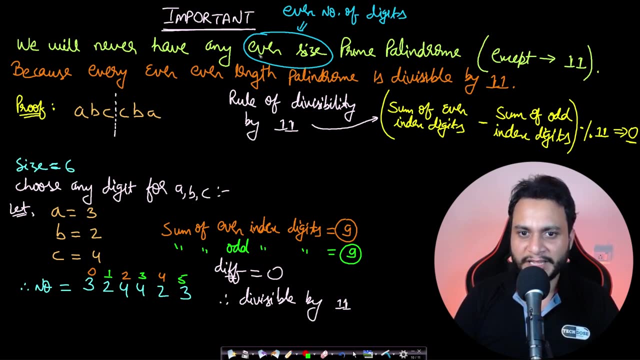 because root n is much larger as compared to log n. now, before we actually move on to the solution code, there is a very important point to consider. like we will never have any even size prime palindrome. even size means even number of digits, except for 11, because every even length palindrome 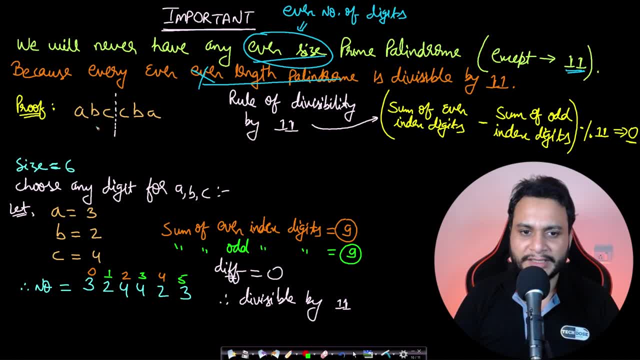 is divisible by 11. let's suppose that we are taking six digits, which is even number of digits, and if i can represent the six digits in this way, is such that we want to make a palindrome: a, b, c, taken on the left side, c, b, a taken on the right side. this constitutes: 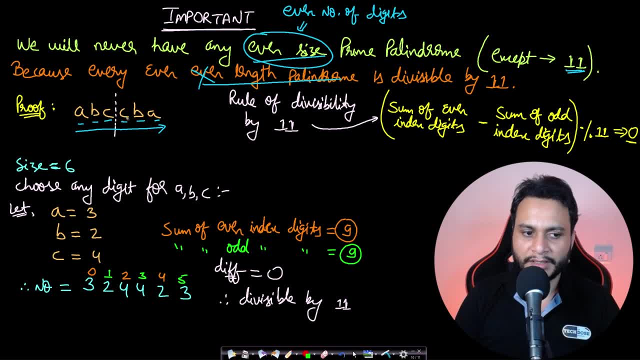 this is the number that would be divisible if the sum was more divisible than 11. and now we are contrelecting it because the out some better ruler says that the sum is divisible by 11är. and okay, one of the other rulesType, выб då and make sure that the sirc is a palindrome. 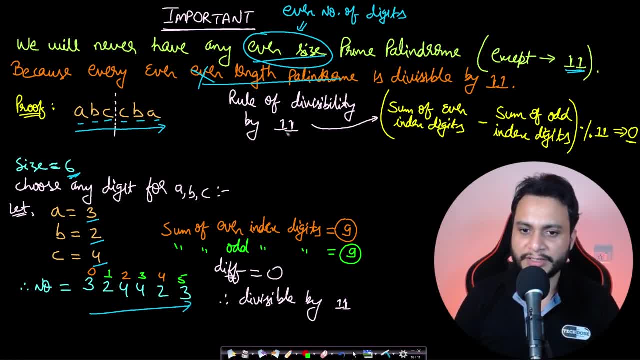 and we are free to choose any of the values for any of these three digits: ABC, let's pick. A equals three, B equals 2 and C equals four, and this is how the number is formed, as we should know, the rule for checking the divisibility of 11.. 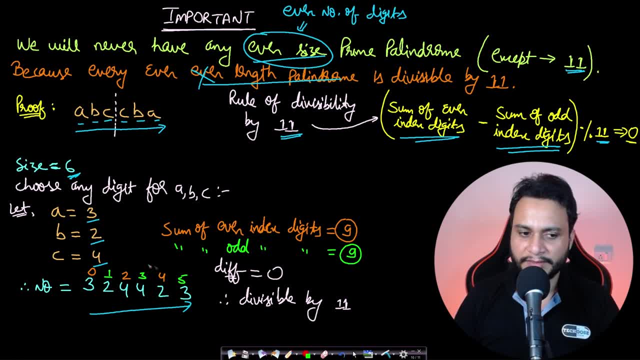 So the sum of even index digits minus the sum of the odd index digits, if it divisible by 11, then numbers divisible by 11, otherwise it will not be divisible. otherwise, if it divisible by the sum, it will not be divisible visible by 11. in this case, if you form an even length number which is a palindrome, the difference, 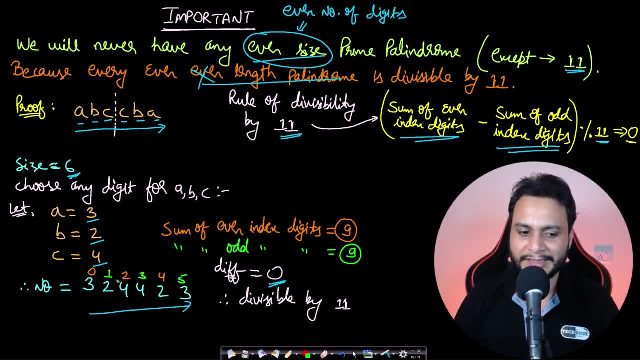 will always be 0. okay, in this case, the sum of even index digits, like 3 plus 4 plus 2, will be equals to 9 and the sum of odd index digit, that is, 2 plus 4 plus 3, which is again equals to 9. 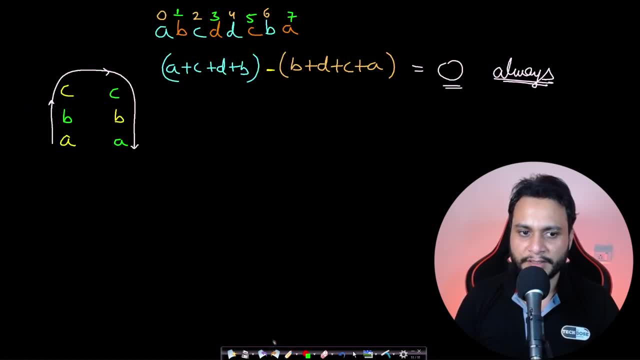 so if you take the difference it will be equals to 0 right, and this is true for any even length digit. you can also think for the eight digit number, which is abcd, separated again dcba, just in the opposite order, and we can pick any of the values. in general case you can just add the even. 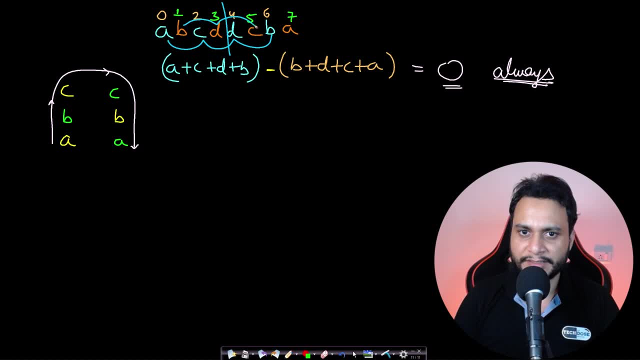 index digits and you can add the odd index digit and if you take the difference, it will always be 0 because each of the pair will get cancelled out. you see, all the pairs are present here, so they will get cancelled out and the answer will be 0. so 0 is divisible by 11. therefore we can. say that any even length number which is a palindrome will always be divisible by 11.. and since prime palindrome of even length are all the subsets of even length palindrome, therefore the prime palindromes will always be divisible by 11.. i would like to announce about our live. 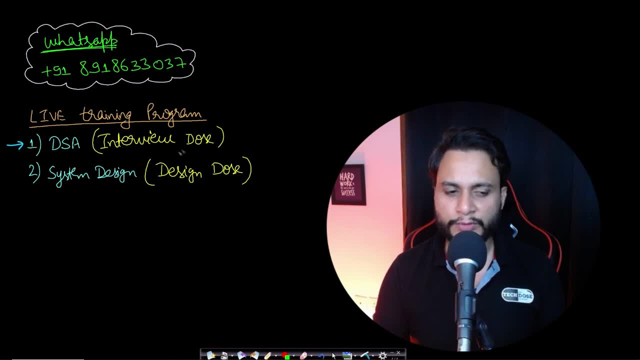 training programs, data structures and algorithms, which is interview dose. and system design, which is design dose. if you are looking for making a switch from service to product based or even switch, and aiming for your dream company, this is the best curriculum you can ever join. i'll be your. 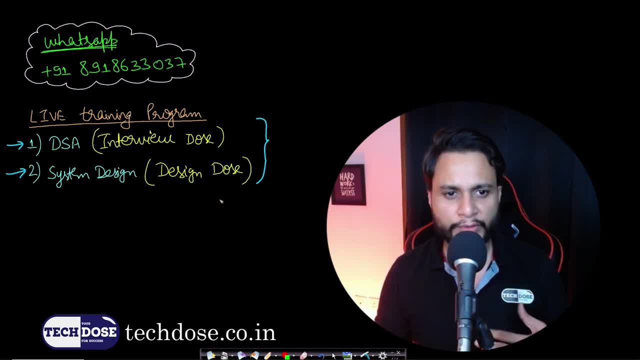 mentor throughout the cohort and i will help you clear all your doubts in the one-on-one sessions. you can know more about this by querying us on the whatsapp number, or you can also visit our website, techdosecoin. let us now look at the code. this is the main function for our code, which is the. 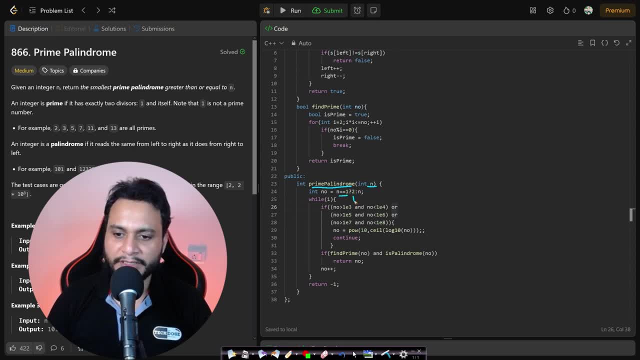 prime palindrome. in this case, we are given the number n. if n is 1, then our answer will be 2, otherwise we will start processing the number. so this is the process and this is the infinite loop. i will be skipping all the even length. number of digits. how? 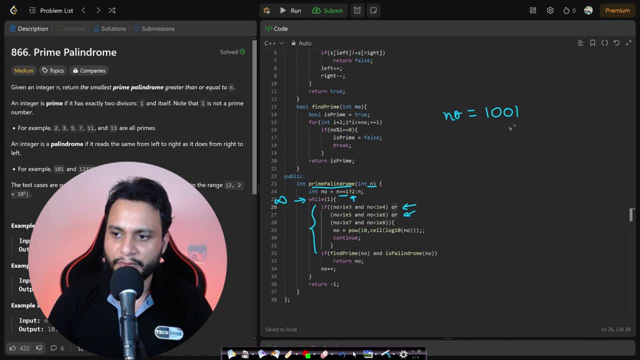 do we do that? let's say the number is equals to one double zero one. so i want to skip all the four digit numbers now. so i will directly jump to the five digit number, and the five digit number the nearest one will be 10 to the power of four. how do we do that? we find the log base 10 of this.